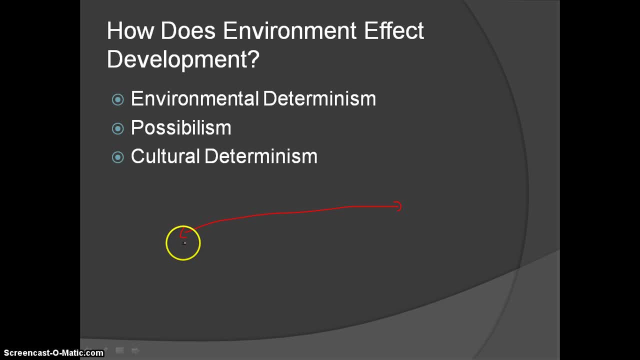 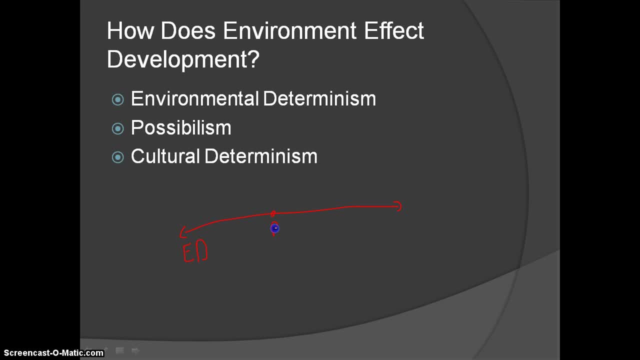 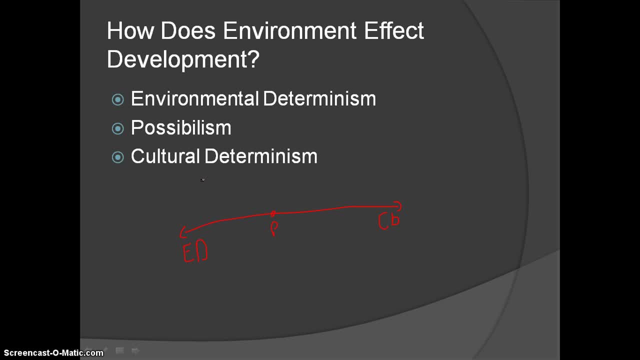 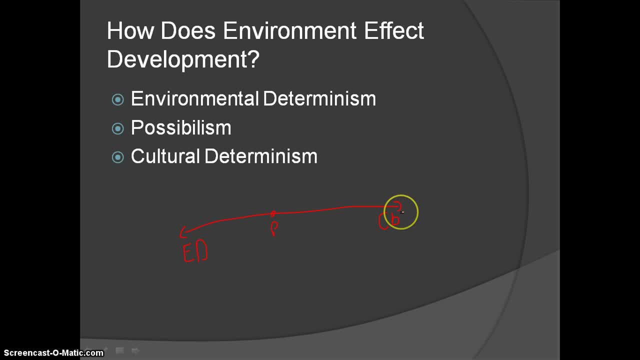 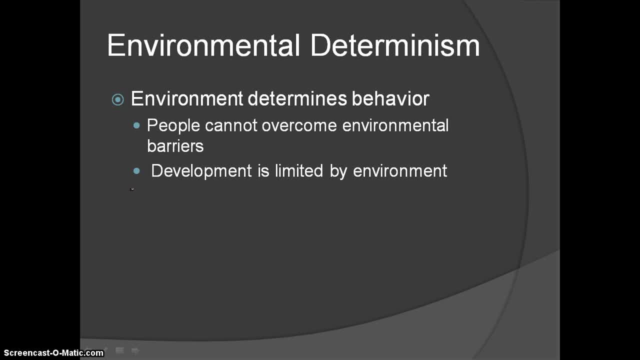 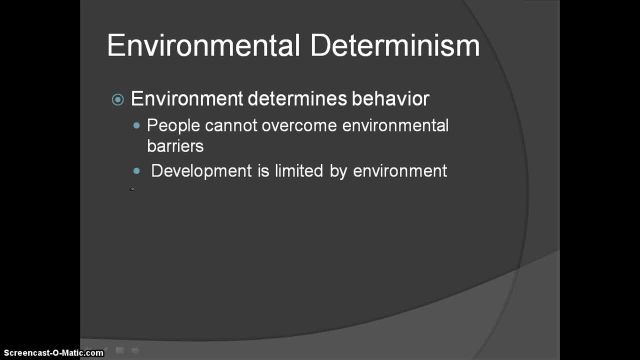 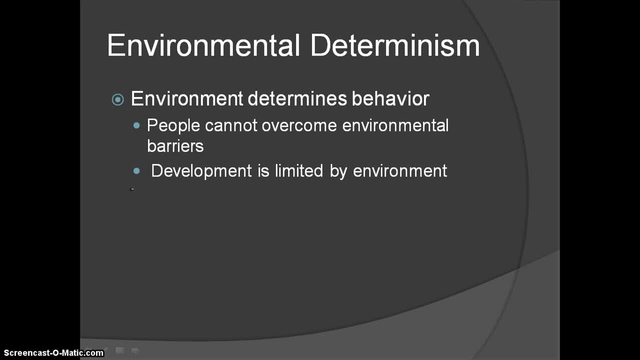 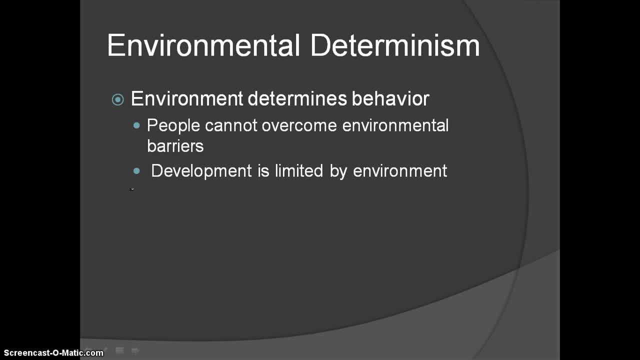 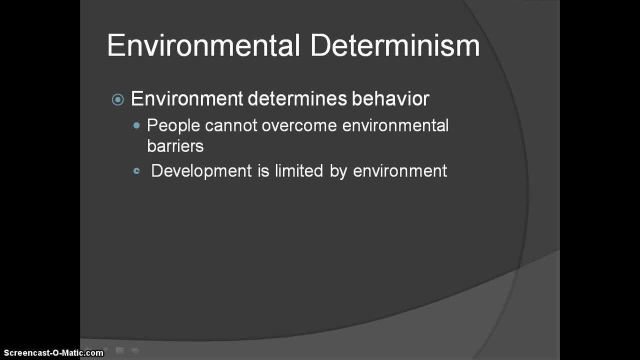 Thank you for watching. Thank you for watching. Jared Diamond, of course, went and looked at the people of Papua New Guinea, and one of the conclusions that he comes to about this idea that they call cargo was that they just didn't. they simply did not have the natural resources necessary in order to develop. 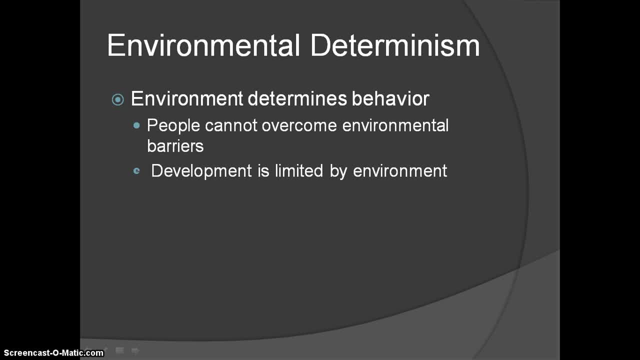 into a more developed, more advanced society, especially things like iron ore to make iron tools, and also the different types of crops that were necessary to sustain larger populations. And so that's kind of his outcome is that because the people of Papua New Guinea had 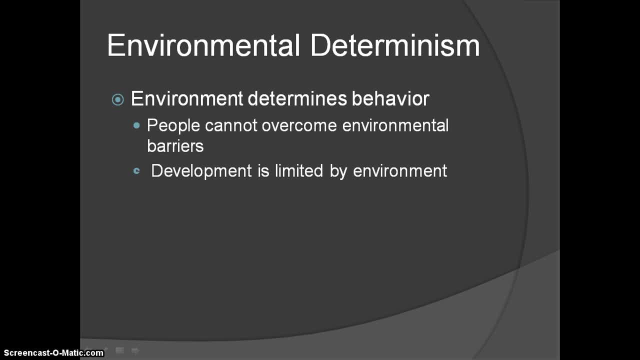 no way of getting these things and really there was no way for them to develop into a more advanced and wealthy society. And so, of course, this idea of environmental determinism. you can kind of see it in a historical sense. You think about the different people across the world and you know, prior to trade and 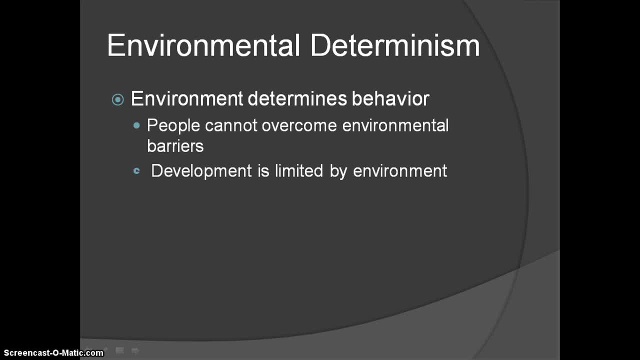 prior to global interactions, and of course it would make sense that people had difficulty overcoming some of their environmental barriers, And they could only go so far, especially if the environment they were living in was particularly harsh. This helped the Europeans to kind of come to some of the conclusions about why they 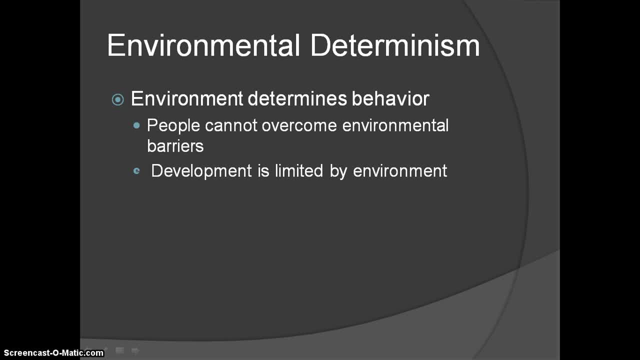 had developed and advanced and some of the people in the tropical areas, parts of Africa and the Caribbean had not. Adam Smith talked about South Carolina being the perfect place for government, and the Europeans thought that the climate, the temperate climate that they had, were much more beneficial to. 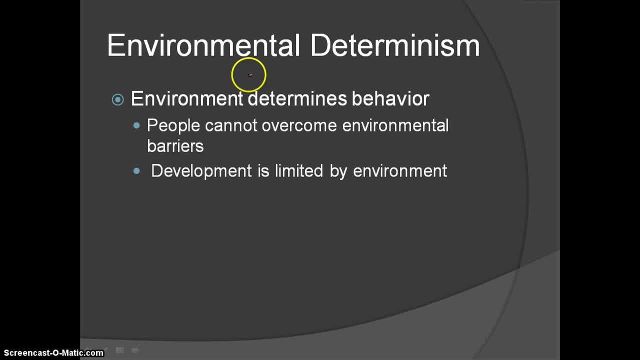 industrious and business and things along these lines. So again, kind of in a historical sense the environmental determinism theory makes sense because there wasn't as much global interaction. So of course people living in harsher conditions are going to have difficulty overcoming them. 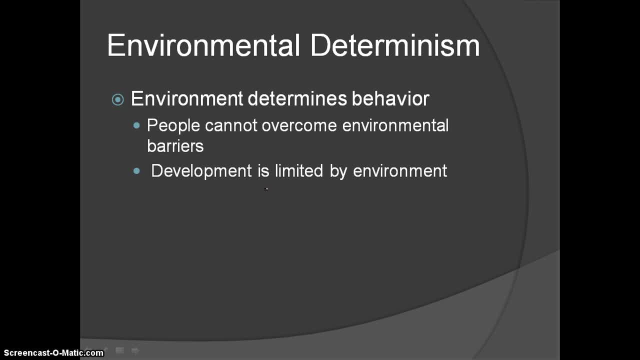 If you think about the things that people use for clothing, for food, for housing, before global interaction and global trade. of course, the things that they are using are going to be limited to the resources that are nearby and available to them. The next step is what is called possible-ism. 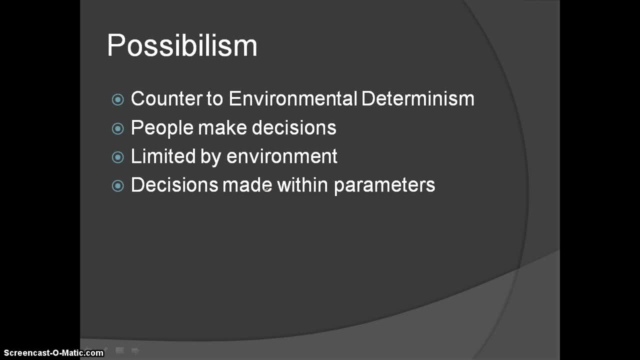 So possible-ism is developed as a counter to environmental determinism, and it's a little bit more positive in that. what it says is that, yeah, the environment creates some sort of limitations, but people are able to make certain decisions that will help them overcome the environment. 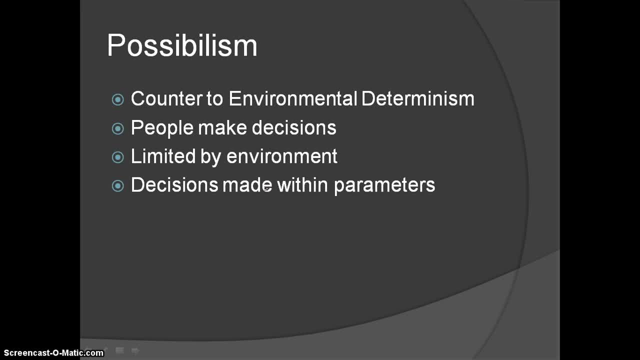 So this allows for some human development, some human advancement. people are interacting with the environment. People are able to change it and to make it work in their favor, But these decisions that they're making can only be made within certain parameters, and so it still recognizes the idea that there still are certain limitations put on people. 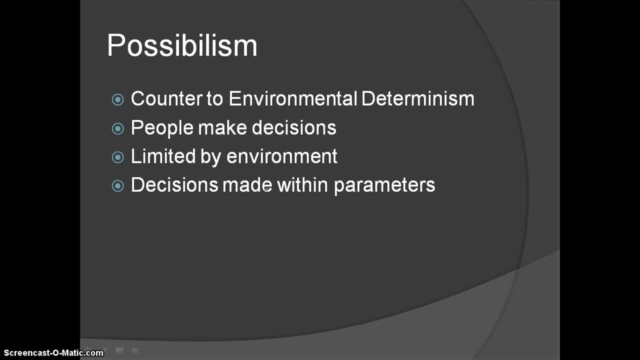 by their environmental factors. So, even though they can make some changes, make some decisions, there's going to be some certain limitations to that because some environmental barriers might be too difficult to overcome. You think about tropical climates, You think about the desert. 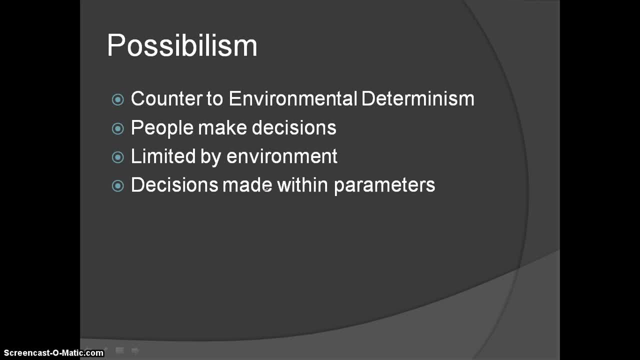 You think about the diseases that are more prevalent in those areas, much more difficult to overcome, especially if we don't have medicines to take care of them. You think about tropical climates and very hot, dry climates, the difficulty of overcoming those conditions to grow enough food for your population. 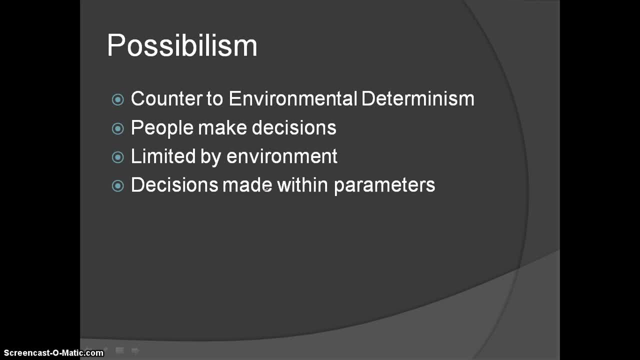 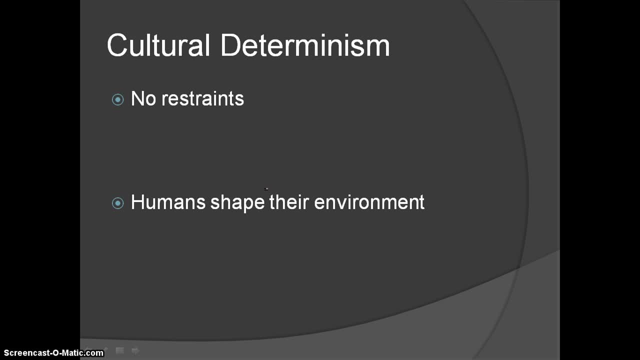 So it would make some sense within, kind, of those frameworks or those particular conditions. Then there's this idea of cultural determinism. This is a much more positive outlook on life and on people and their situation. Basically, cultural determinism says: look, there are no restraints on people and the advances. 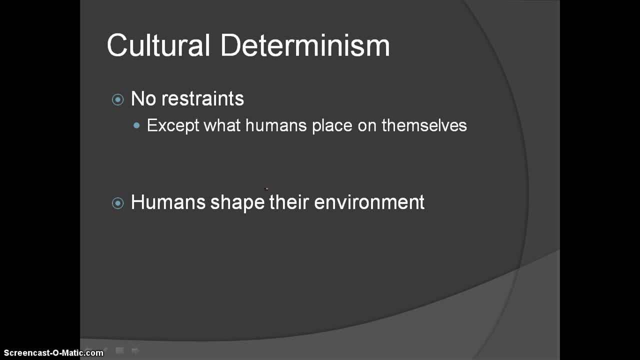 they can make on society. Basically, it's just this idea that there are no restraints, except what restraints people put on themselves, And this is going to be based upon their culture. So if their culture decides for them, what is it that will and will not be acceptable? 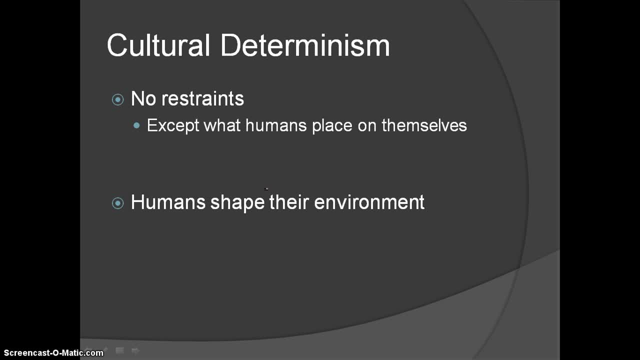 you think about. I made mention of this, I believe, in my last video. You think about Islamic and Jewish traditions not wanting to eat pigs. it's not because pigs weren't there, it's because they were considered to be unclean animals. You look at some Islamic countries in terms of their view of women and how women should. 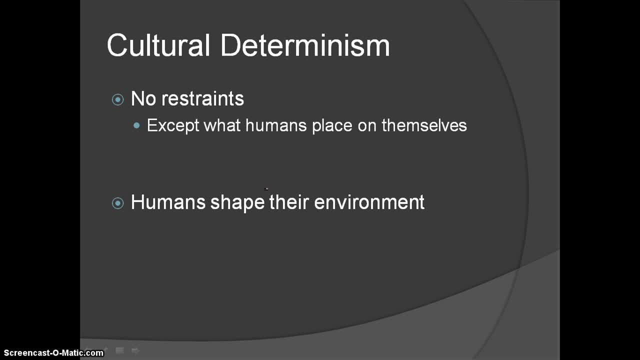 behave in public. So that's what's going to keep their society from moving to a freer society where women are able to more fully participate and might even hinder their economy. Humans are not able to have the best and the brightest involved in those types of things. 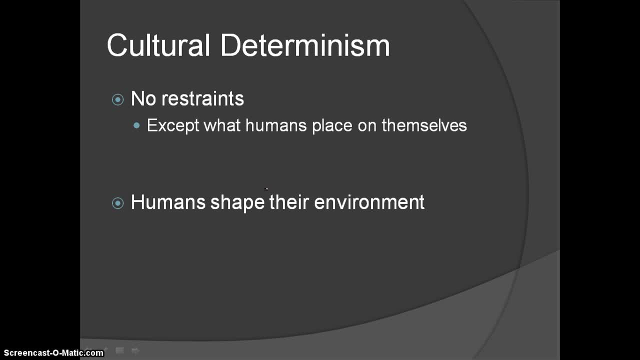 So the culture is what's going to be holding those people back, holding their societies back, and not necessarily the environment itself. Again, it's this idea that these restraints are not environmental restraints, rather they are cultural restraints, And so humans are going to shape the environment, no matter what. 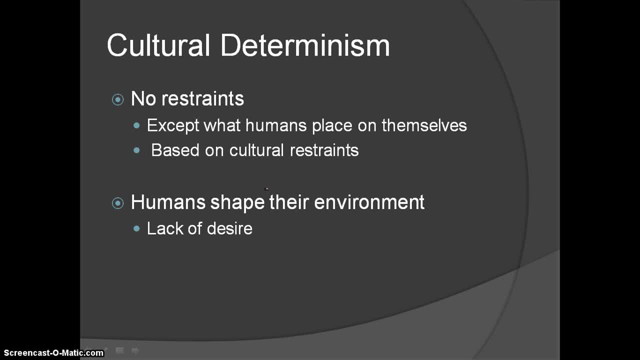 But basically the only restrictions are going to be some sort of lack of desire to shape the environment In the way that might be helpful to them. And I mean this could be any lack of desire, whether it's a religious lack of desire. maybe there's some sort of moral restraint. 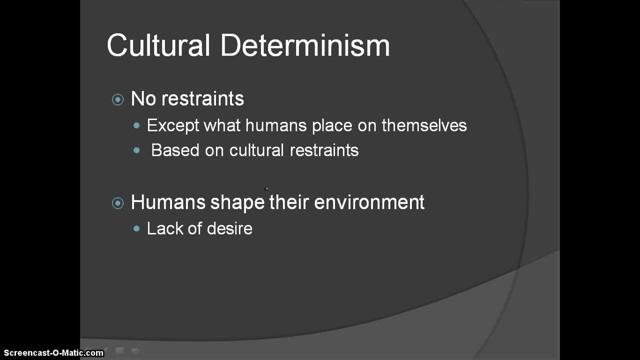 You know, even in the United States there are certain places that we consider to be off limits. Redwood Forest. we're not going to cut that down just to make more room for houses. We consider that to be a place that should be preserved, and so even our culture values. 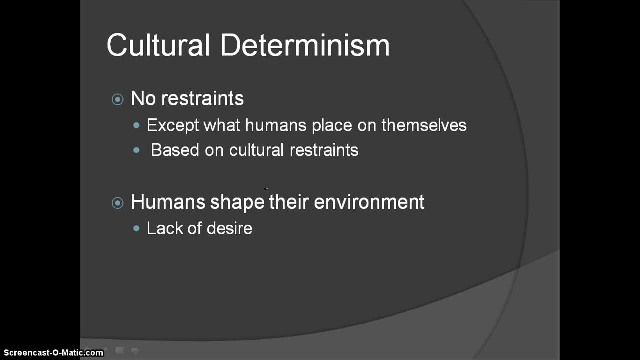 some of those places And things like that, so we're not going to infringe upon that. Now, within cultural determinism, one of the things that's absolutely necessary is advanced technologies to allow us to overcome some of the environmental barriers. So, if you look at possible-ism, one of the reasons that possible-ism comes about is because 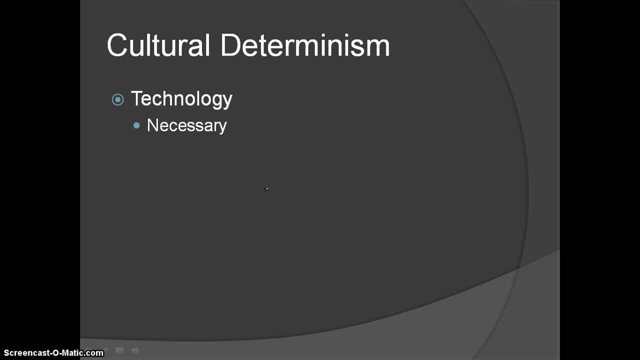 some of the technologies are not available. Well, now that we have technologies that allow us to do things like fracking to get natural gas and oil in places that previously were not available to us, Our ability to build cities and roads and place infrastructure in places that in prior 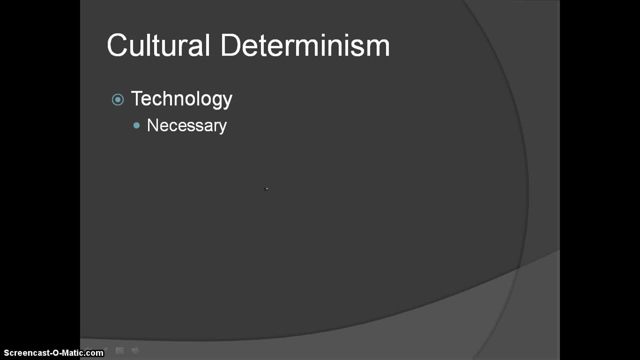 years were, it just was unthinkable- this whole idea of hydroponics and growing plants and water and being able to turn places that were infertile into fertile areas, and the new hybrid plants and new seed technologies that we have out. So things that before seemed absolutely impossible are now possibilities. 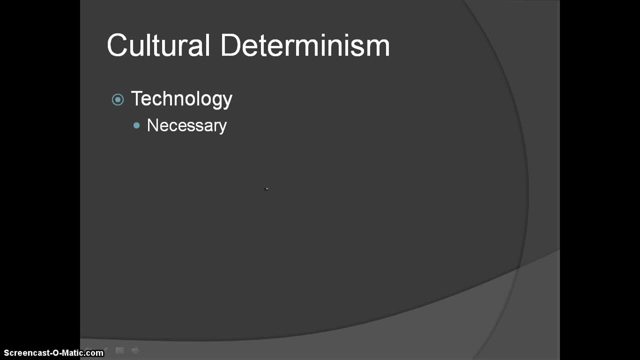 And that's what we're going to do And helping us to overcome some of those environmental restraints, and so that's really helpful with cultural determinism And so you can see how this progression takes place, especially over time, as new advancements are made, and then, you know, it helps us to get kind of a different picture of what people 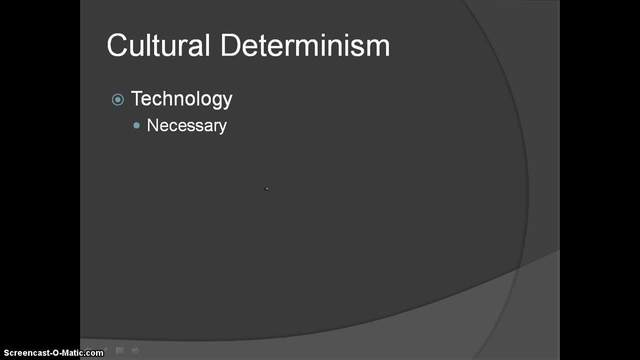 are capable of. All right, so that's it for this time. Thanks for listening and come back next time when we're going to come. we're going to talk about some of the specific elements of culture. Bye, Bye.